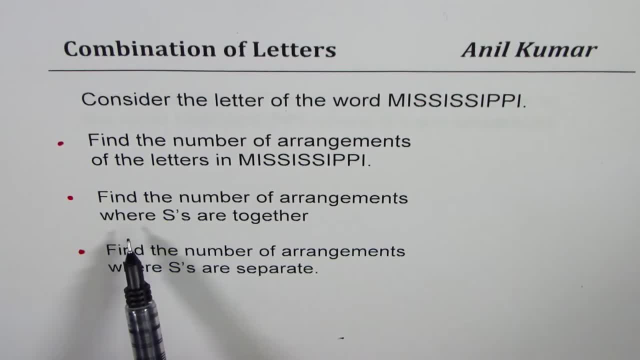 And then we have a conditional statement which says: find the number of arrangements where S's are together. In Mississippi there are four S's. We want all of them to be together, And the last one here is: find the number of arrangements where S's are separate. So that's the question. 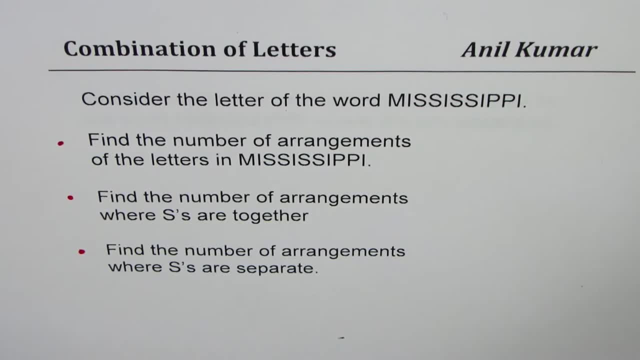 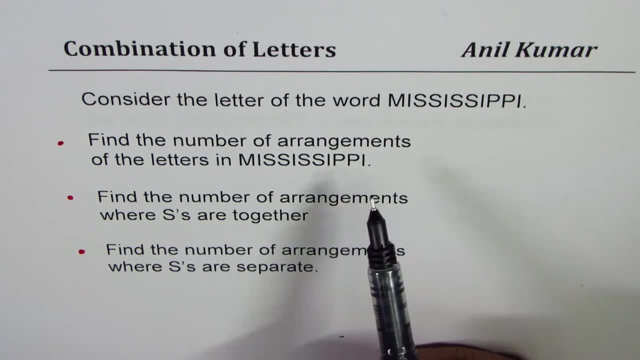 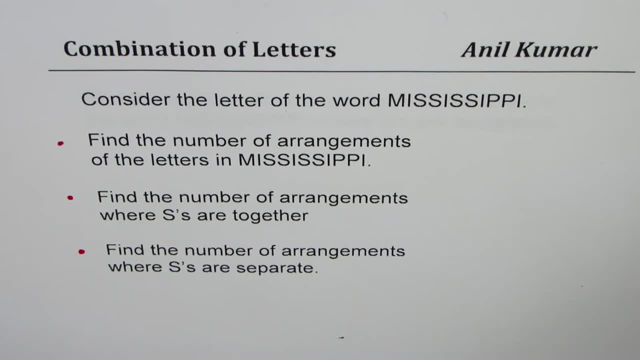 what we do is we just count how many letters are there. In Mississippi we have 1,, 2,, 3,, 4,, 5,, 6,, 7,, 8,, 9,, 10, 11 letters. So let's write down: we have 11 letters. Okay, Then we look for more than. 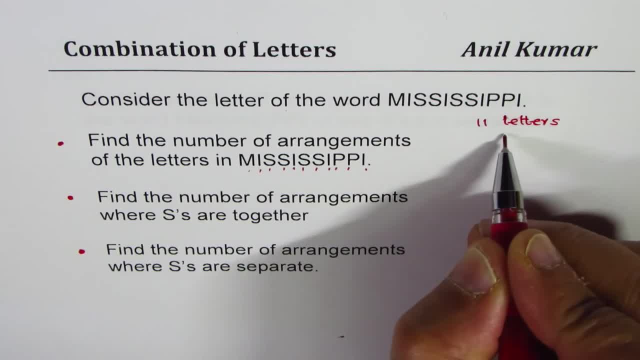 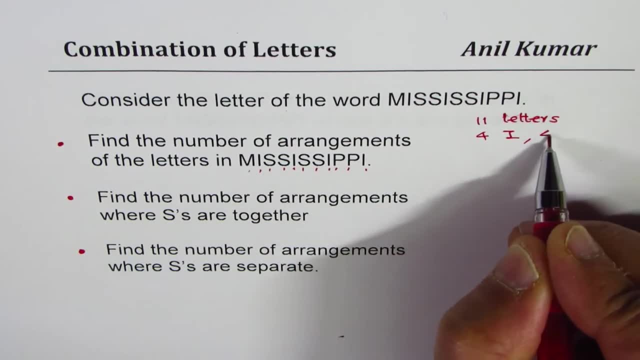 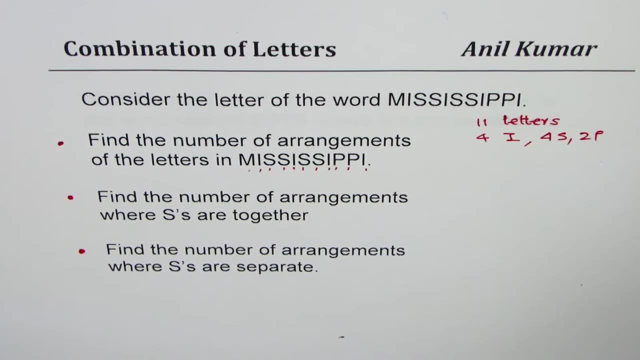 1, which are repeated I's. So I's are repeated. How many? I's? 1,, 2,, 3, 4.. Then S, We have 4 S And we have 2 P's. Now this is a very special word which we always talk about when we have. 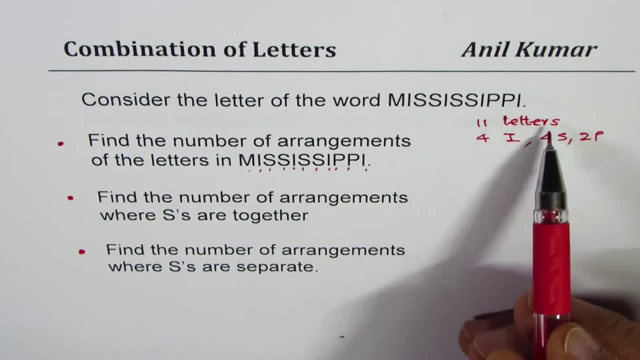 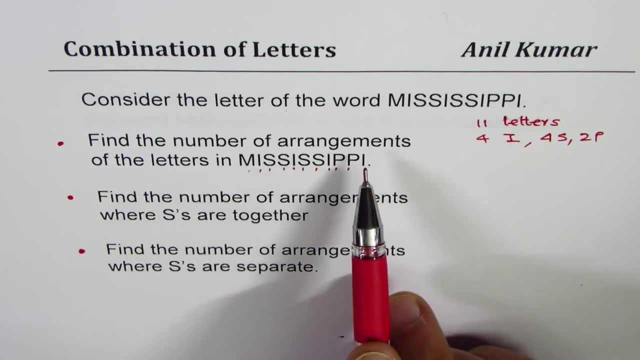 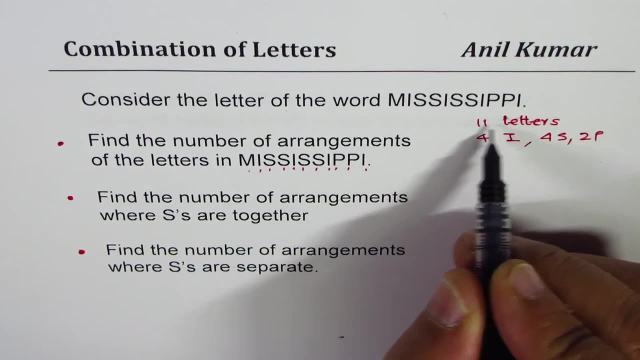 this kind of a question, right? 11 letters, 2 I's, 4 S's and 2 P's. Now we need to find the number of arrangements for all these letters. So the answer is, as most of you know, 11 factorial. 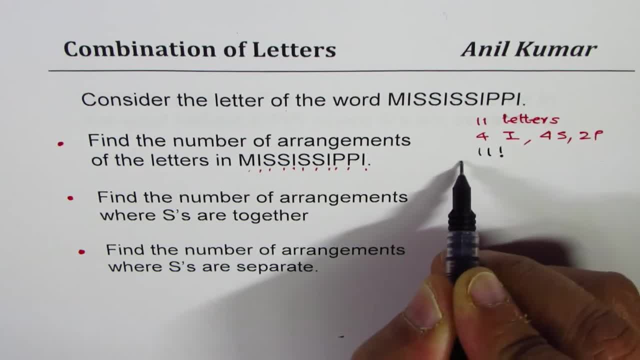 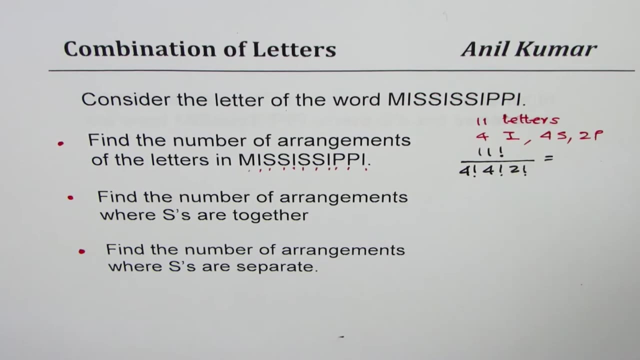 total combinations divided by how many are of the same kind: 4 of I's. so divided by 4 factorial, 4 S's 4 factorial, 2 P's, 2 factorial, correct? And you get your answer. So that's the first. 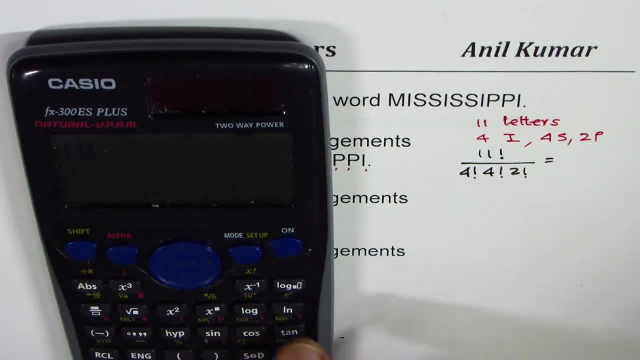 answer. So we have 11 factorial divided by within brackets, let's say 4 factorial times 4 factorial times 2 factorial right Bracket close equal to the answer is 34, 650.. Correct The next one. 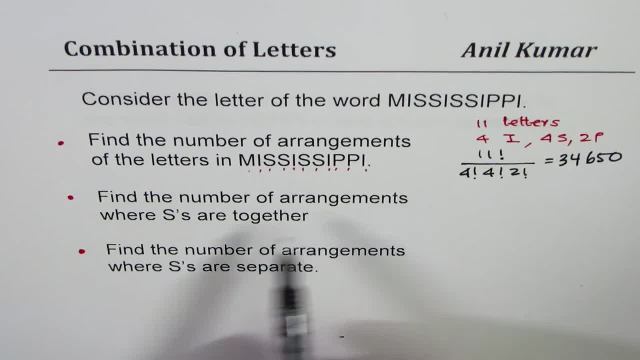 here is: find the number of arrangements Where S's are together. Now that's kind of tricky. What do we do for doing or solving such questions? Now, when we want to put S's together, we rearrange so that we take away. 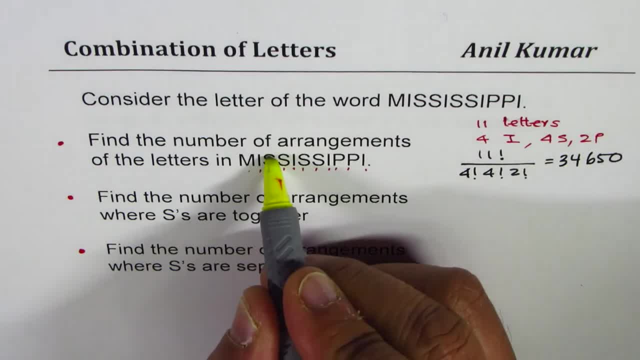 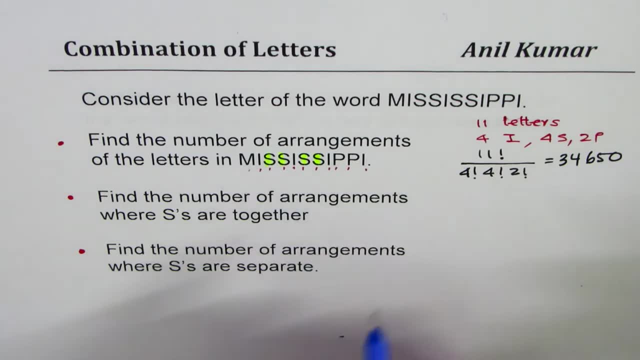 these S's and group them together. So these are the 4 S's. So let's write down the word once again, And this time let's put S's together: 4 S's. Let's take them to occupy one space. The rest of the letters are M. I let me write. 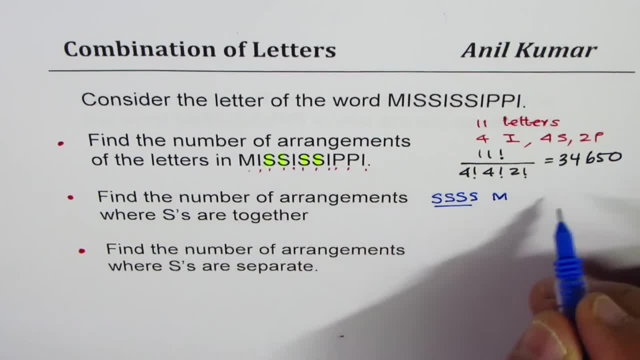 down M. then we have 1,, 2, 3. I's 1,, 2,, 3, I's 2 P's. You could have written 4 together. anyway, These are the other letters. We want all S's to be together, So think as if this: 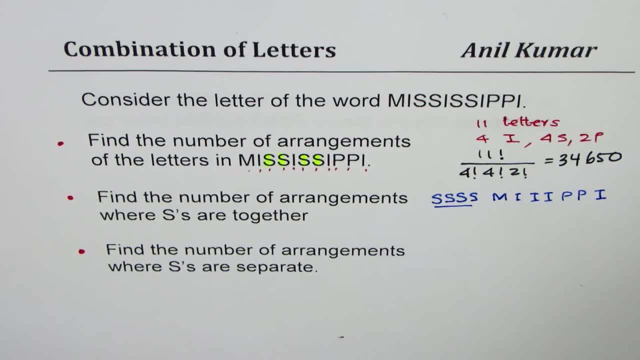 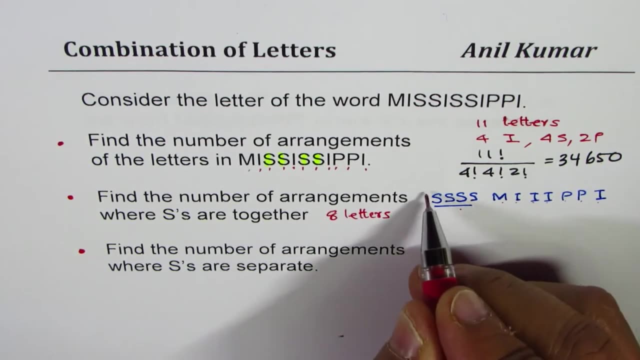 is one particular group, Right, All S's. So what do we have here Now? we have 1,, 2,, 3,, 4,, 5,, 6,, 7, 8 letters. Do you see we have 8 letters? We are considering this to be one group, So one letter S Out. 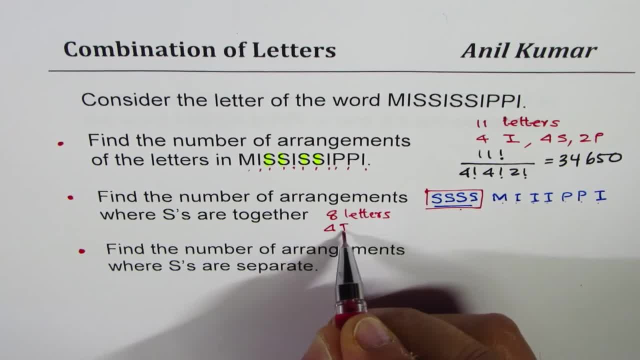 of which 4 are I's and 2 are P's right. So how many words can you form? M I? 2, 3, 4, 5, 6, 7, 8.. Meaningful or meaningless? Well, the words will be, since there are total 8 letters. 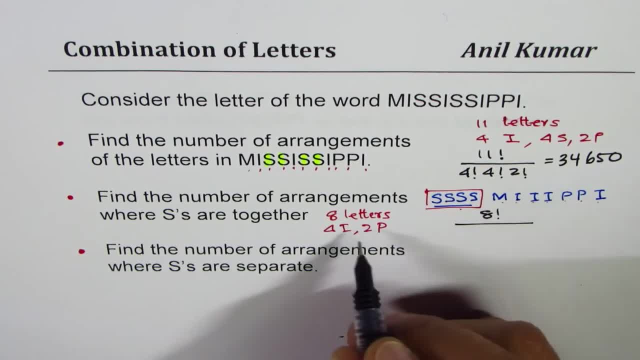 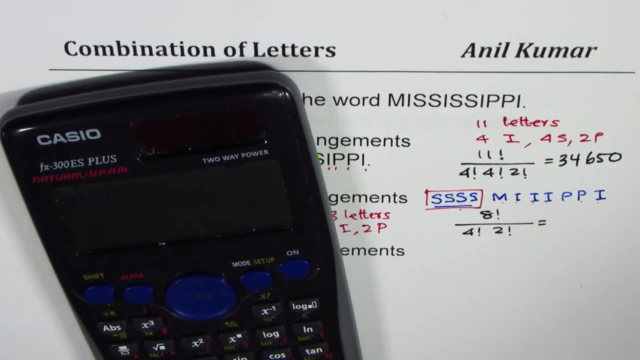 8 factorial divided by 4 factorial for the I's and 2 factorial for P's- Correct. So let's figure this out. We have 8 factorial divided by: within brackets, 4 factorial times 2 factorial- Correct. So let's go ahead and take a couple of steps. 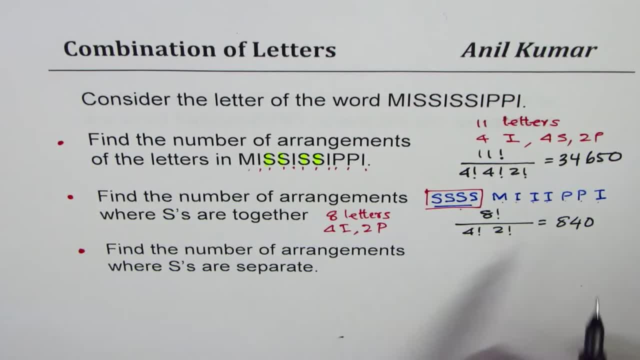 8 factorial divided by 2 factorial- Perfect. Now I'm going to take a few steps. S is now a number of P's and 2 is a number of P's. Let's start. So what are we going to do? Well, we are going to take a few steps. How many I's? and 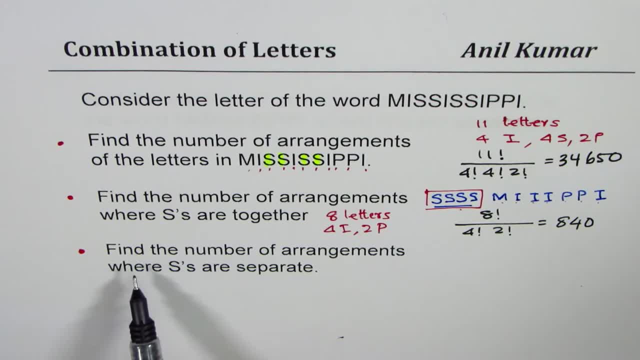 2 factorial. 5 factorial. Oh, 5 factorial. Here are our 4 factorial and 5 factorial is the number of I's and 2 factorial. Yes, here are 7 factorial's. This is the final, final, final step. 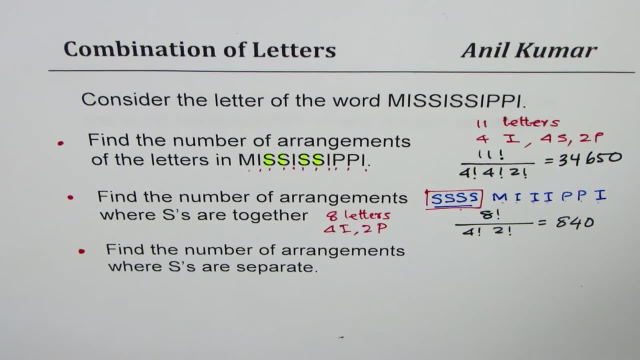 Here are any numbers of I's and 2 factorial. Here are 2 factorial. very tricky. many times I have seen students answering like this: total number of commissions: three, four, six, five, zero, SS together: eight four zero. you take away 840 from 34, 650 to give an answer here. well, that is going to be. 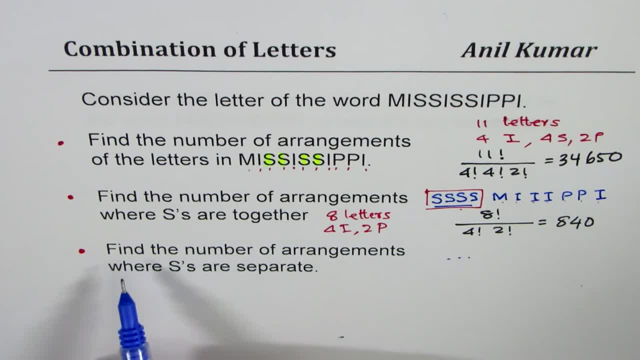 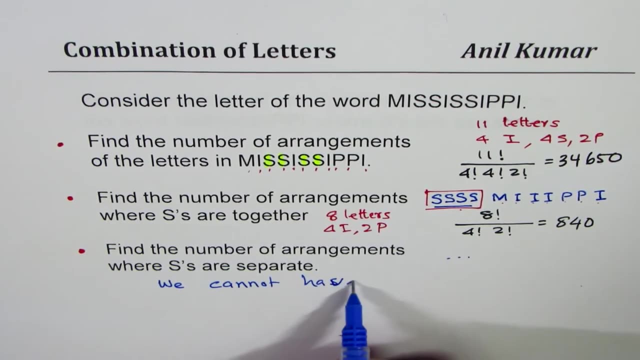 wrong. incorrect reason is: it says: find the number of arrangements where SS are separate. try to understand. s is a separate means. we cannot have, remember this, we cannot have, I mean, have two SS or three SS, do you see that? or four SS. now, if you do 340, 650 minus 840, what you get is which excludes four SS to be 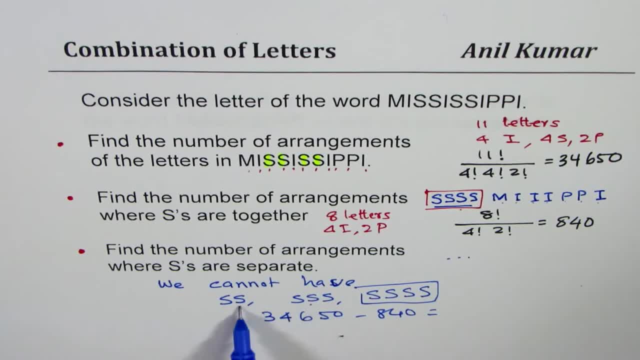 added, do you see that it doesn't take care of other cases? and if you try to solve it using cases, it is going to be kind of tricky, very difficult. so for such questions we'll adopt a different method. right, so we have an alternate way to do. 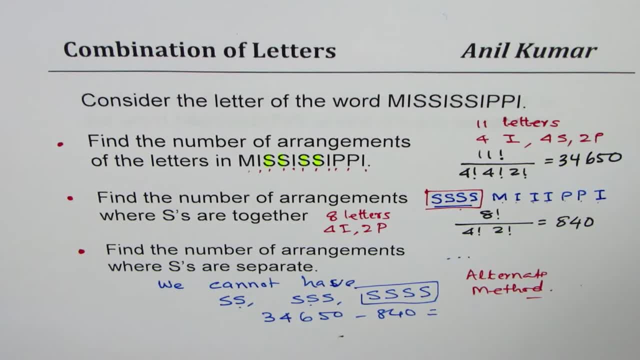 it. let's call it an alternate method, which I'll take up now. so I hope you have understood the idea of this video. these are very common questions. find the number of arrangements of letters in Mississippi straightforward. find the number of arrangements where s's are together, club them and get your answer. 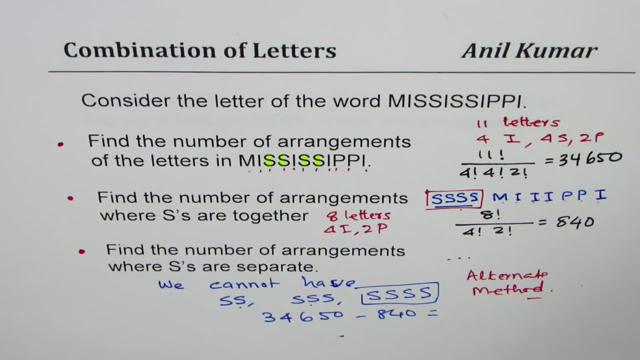 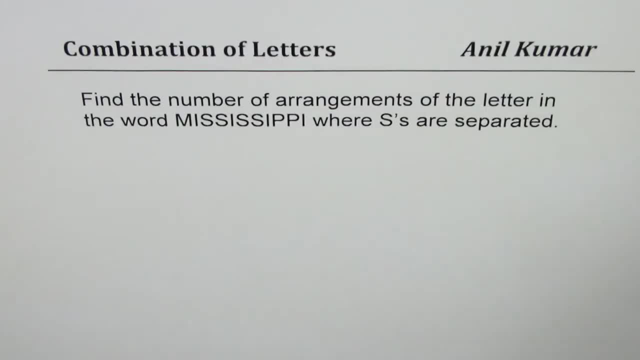 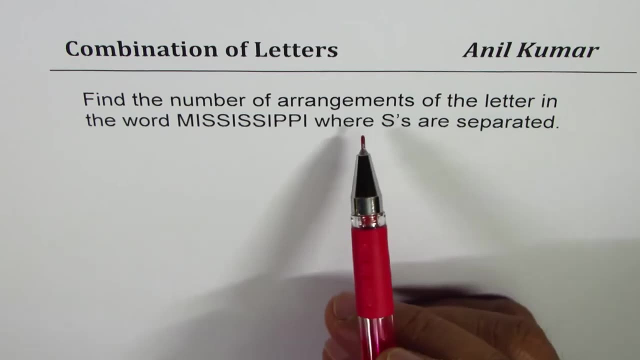 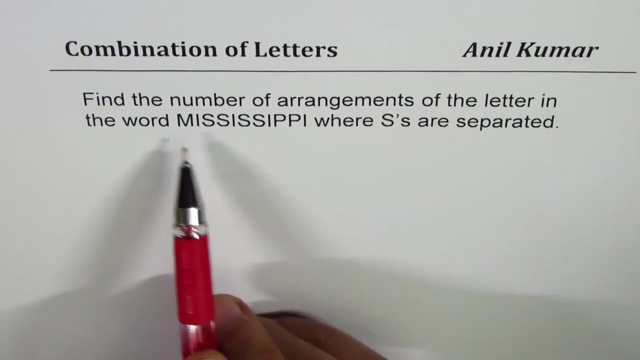 but the real question here is: find the number of arrangements where s's are separate, right? so let's see how to do such questions correct now. so let's look into our third question, which is a major question for this particular video. it says: find the number of arrangements of the letter in the word Mississippi, where 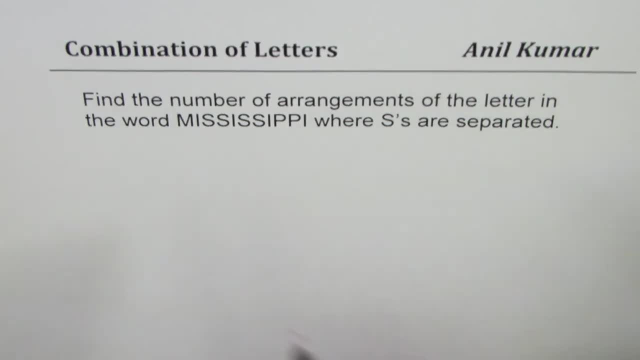 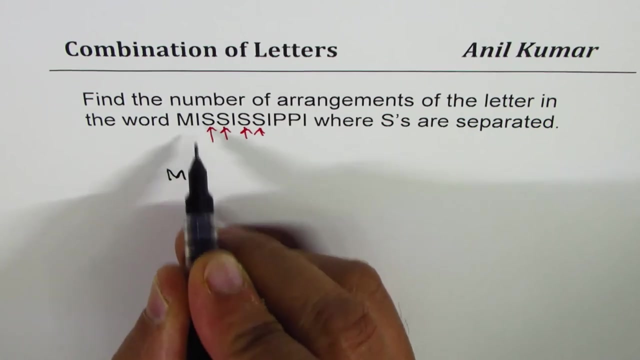 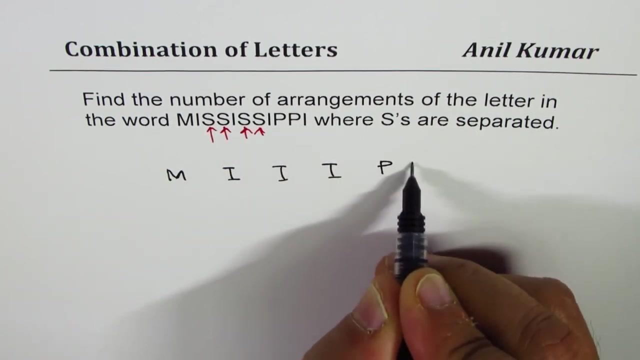 s's are separate. so what we do here is that we take away these s's. so these are our four s's, we take them away from the word. in that case, what are we left with? we are left with M, I, the next, I, another, I double P and I. so we are left with one, two, three, four, five, six. 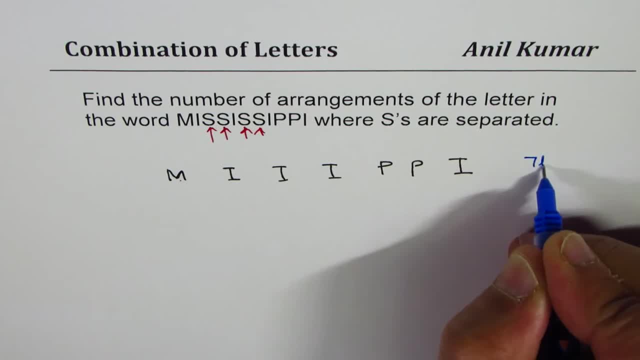 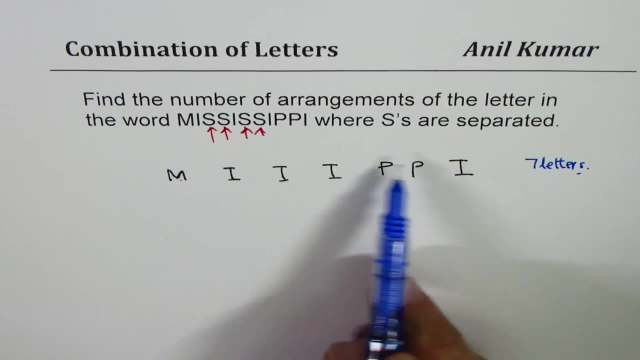 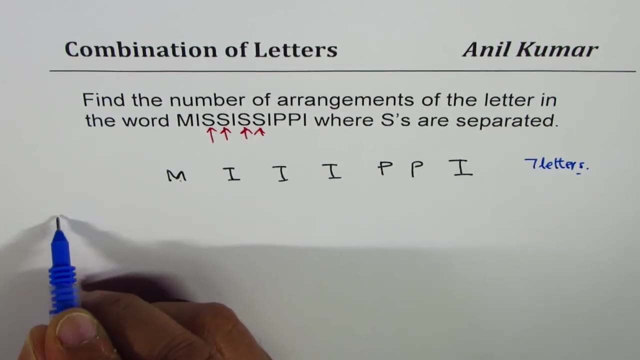 seven, right, so we are left with seven letters. now the idea is: how many words can you make with these seven letters, right? so how many words with seven letters? so now you'll find words with seven letters. now, what you also observe here is that we have four eyes, in which we have four eyes and two peas, so the 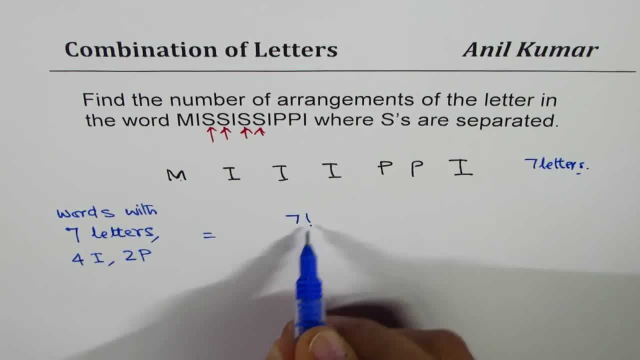 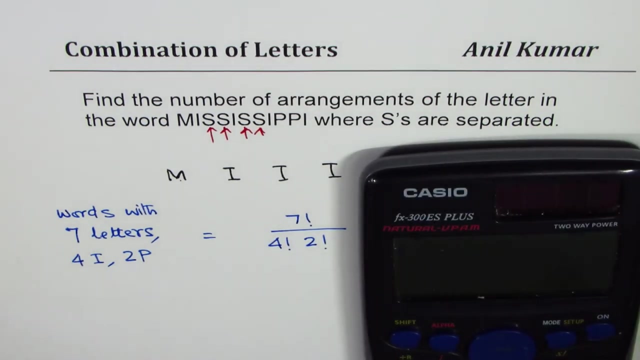 method you knows for several letters: seven factorial divided by repetition of eyes four times, and for peas too. so that gives you the total number of words which can be made using miii PPI. right, that is excluding these SS. let's calculate this value: seven factorial divided by, within brackets, four. 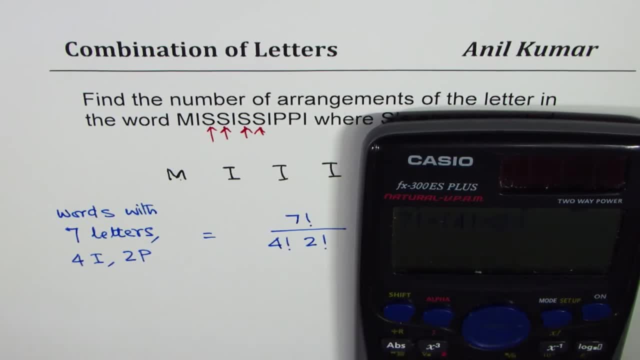 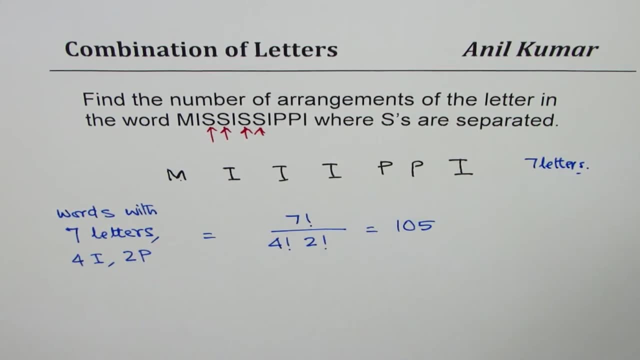 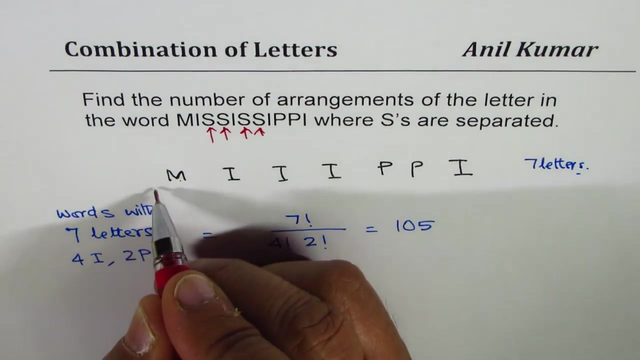 factorials times two factorial, and that gives you 105. okay, so you can make 105 words using these. now what we do is we insert these SS separately so that none of them is together. that's the whole idea. where could you insert? you could start with an. 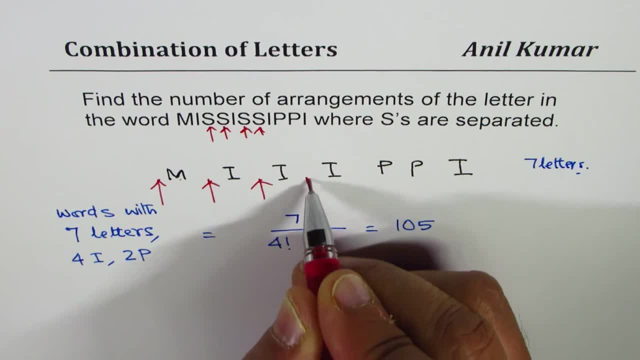 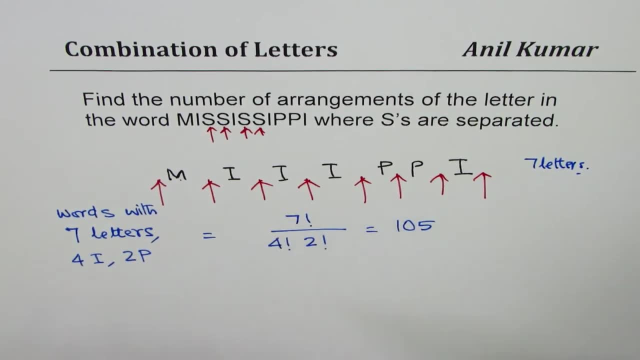 s. you could insert one here, one there. so these are the gaps in the, in the, the in which you can fill up these S's. How many are these? We have 1, 2, 3,, 4,, 5,, 6,, 7,, 8,. 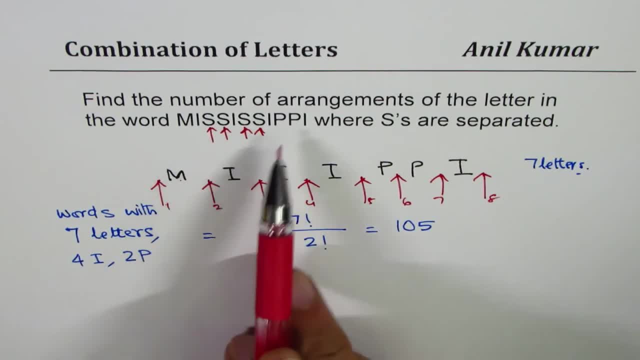 one more than 7.. Do you see that? So we have 4 S's to be placed in 8 positions. So what we have here is 4 S's to be placed in 8 positions. So that gives you how many combinations right. 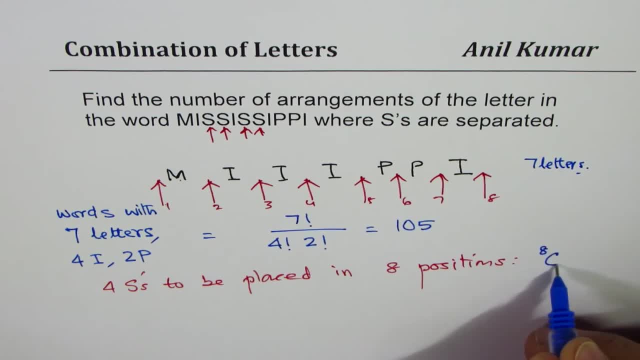 That gives you how many combinations. It gives us 8 C4 combinations. Now these 8 C4 combinations apply to all 105 combinations of S's. These are the combinations of the several letters which we have talked about. So therefore we can now write down that the number of arrangements. 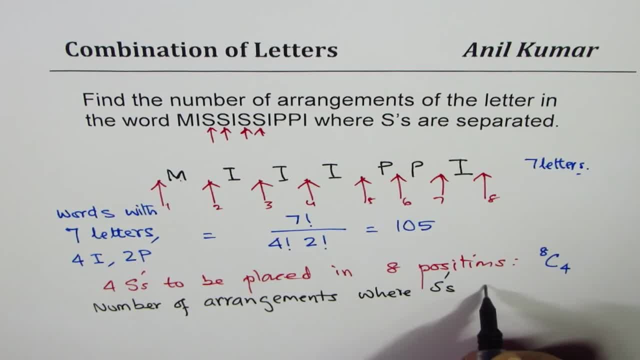 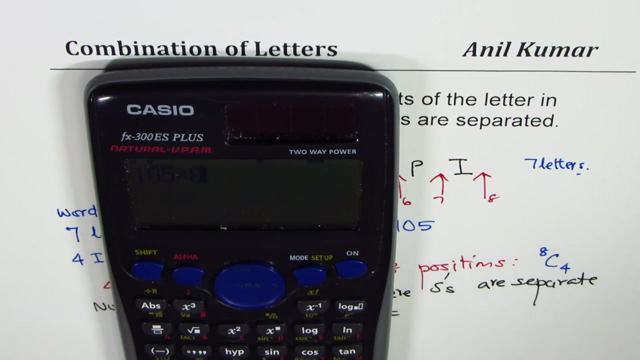 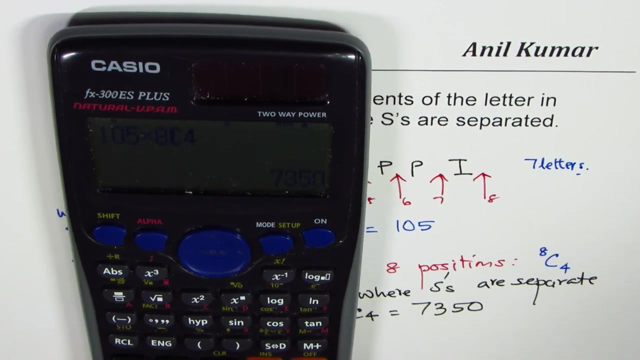 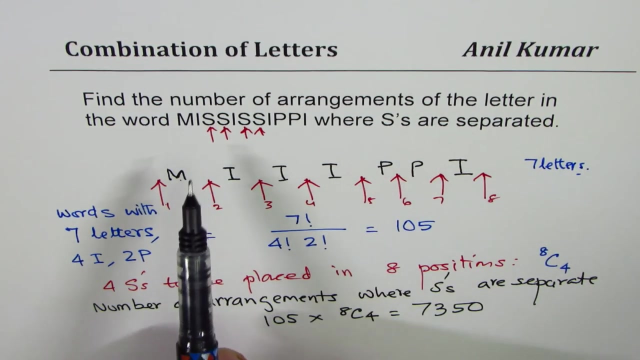 where S's are separate are how many Product of these two, right? So they are 105 times 8 C4, that is what it is. So let us calculate, right, So we will do 105 times 8 C4, and that is 73.50.. So there are 7350 arrangements which you can make with the word. 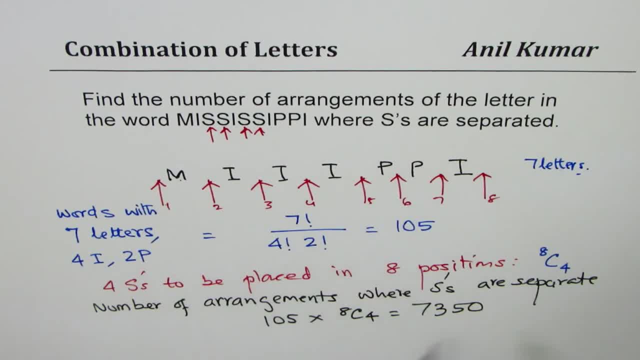 Mississippi, where S's are all separate. Do you get an idea right? So that is how such questions can be answered. I hope that helps. I am Adil Kumar. You can always share and subscribe to my videos. Feel free to post questions. Thank you and all the best.